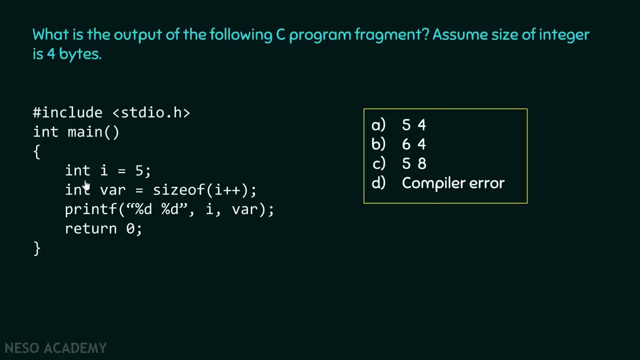 Because i is of integer type. therefore 4 bytes is returned. Right, This is for sure that this particular variable var would contain value 4 after performing this operation. Therefore, c cannot be the answer, Because here the size of this particular operand printed is 8.. 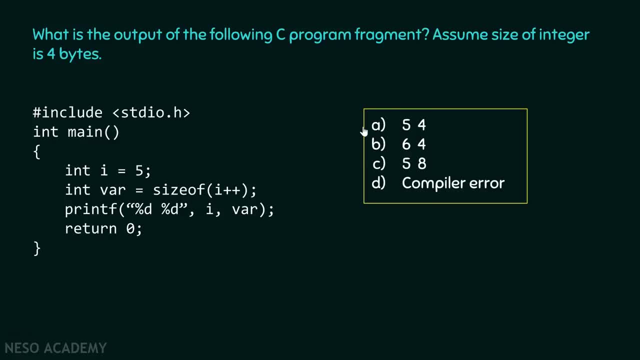 Therefore, c cannot be the answer. It can be b or it can be a. You might think the answer is b As inside the size of operator, this particular expression will get evaluated, that is, post incrementing the value of i. After post increment, value becomes 6.. 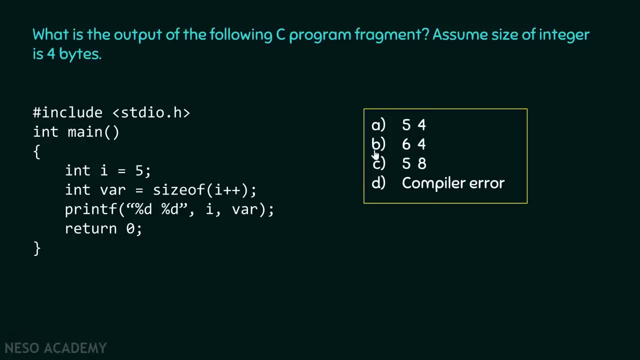 And 6, 4 will get printed Right. No, this is not the answer. Now, this is the one point. we need to understand Why b cannot be the answer. Let's try to understand by considering the original documentation of C99 standard. 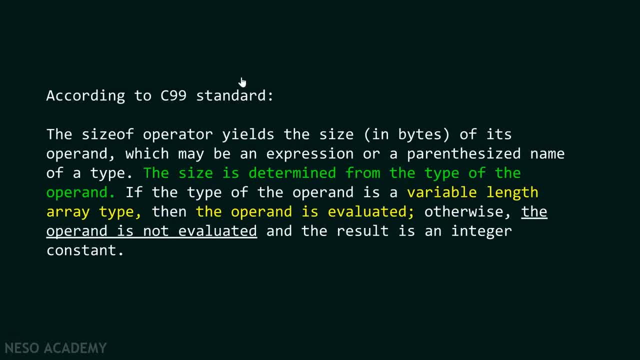 First of all, let's try to understand what a C standard is. C standard is the language specification which is adopted by all C compilers across the globe. Please note down this point. C standard is the language specification. Whatever is provided inside the C standard. 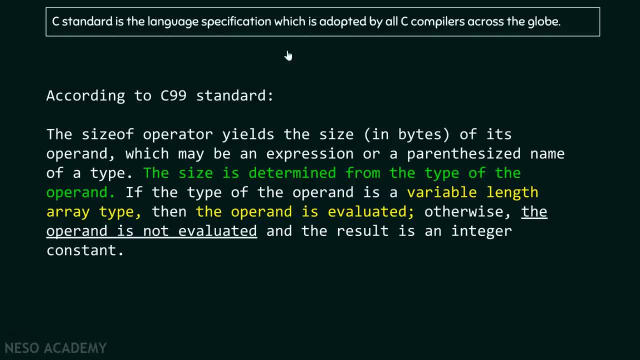 it needs to be adopted by all the C compilers which are available across the globe, Like, for example, inside the C standard something is written about the for loop that explains its functionality. Then all C compilers must have to adopt the functionality of for loop, which is provided by the C standard. 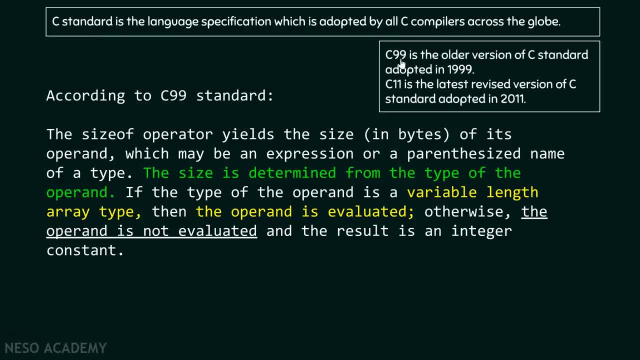 Okay, C99 is the older version of C standard, adopted in 1999.. And C11 is the latest revised version of C standard, adopted in 2011.. Now, according to C99 standard, the size of operator yields the size of its operand, which is in bytes. 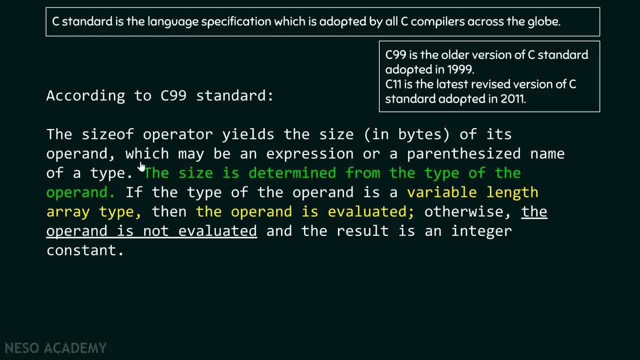 Right, That is the functionality of size of operator, which may be an expression or a parenthesized name of a type. It can be an expression or it can be a type, like int, float, long, double, etc. Size is determined from the type of the operand.